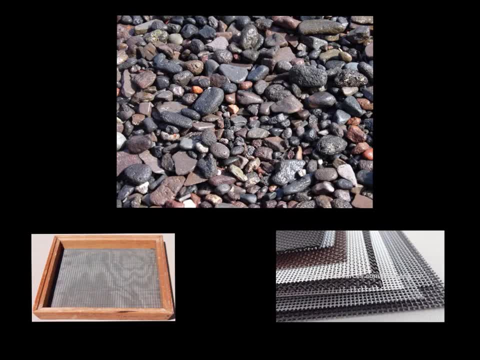 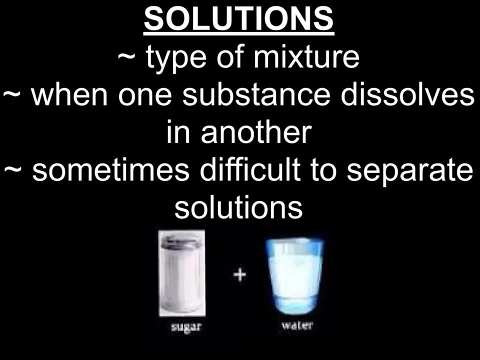 screen to filter out the next size rocks and put them in another pile, And so that's how we would use screens to filter out different mixtures. You are going to add these notes to your note page. So solutions: they are a type of mixture. Solutions are when one substance dissolves in another. 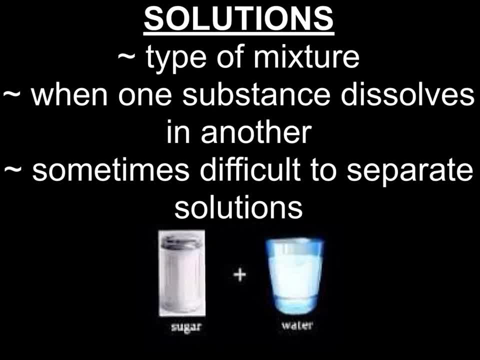 And then sometimes solutions are difficult to separate. So one example of a solution that's very common is sugar and water. When we dissolve sugar and water we can't see the sugar particles anymore. It's evenly distributed throughout the water particles, So that makes it a solution. We. 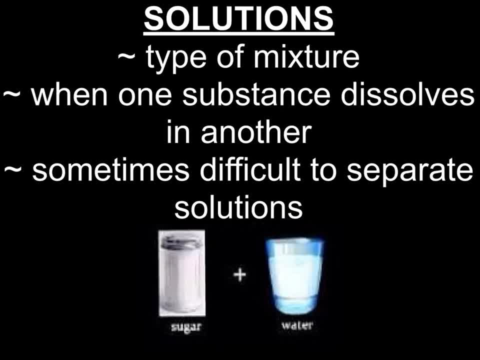 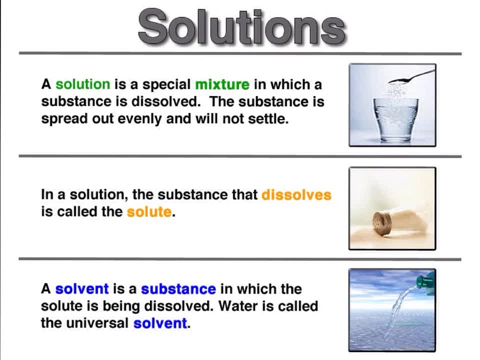 only know that there's sugar in the water when we take a sip of it and it's sweet. So here's some more specific information about solutions. A solution is a special mixture in which a substance is dissolved. The substance is spread out evenly and does not settle at the bottom. In a solution, the substance that dissolves 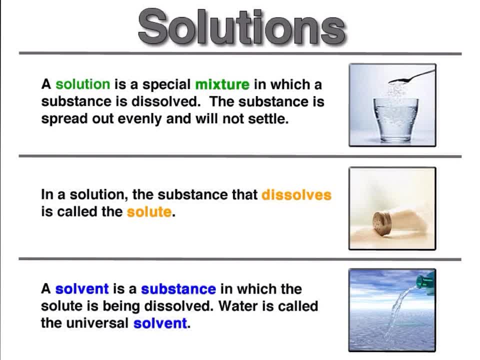 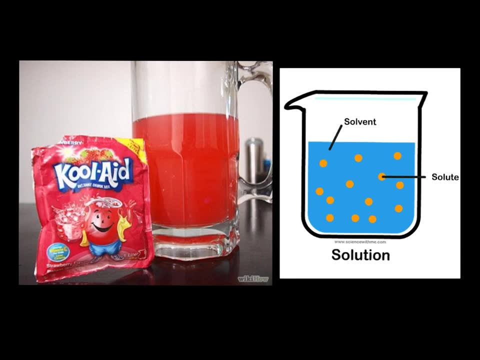 is actually called the solute, And then a solvent is a substance in which the solute is being dissolved, So they tend to think of water as the universal solvent. so kool-aid is an example of a solution. the kool-aid mix, which would be the solid, is the 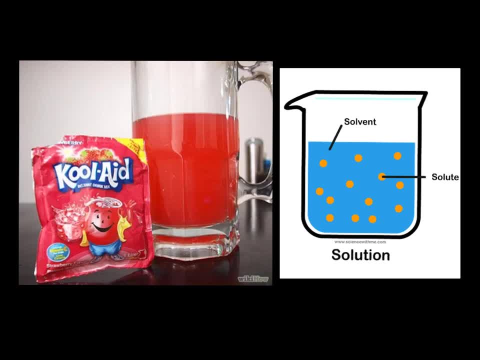 solute and the water is the solvent. and when we mix them together, the solute of kool-aid dissolves in the water and we can't see the different particles. it looks like one substance. other similar examples would be making lemonade, coffee, hot chocolate, etc. etc. 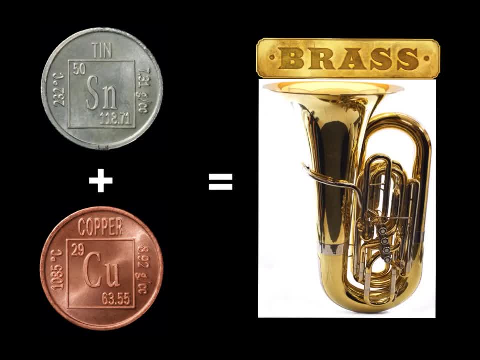 so I can make a solution using two solids also. I can take tin a solid, I can take copper a solid, and what I would do is I would melt both of them and then I would mix the melted liquid and that would make a solid brass once it hardened. so I can take two solids and also mix them.